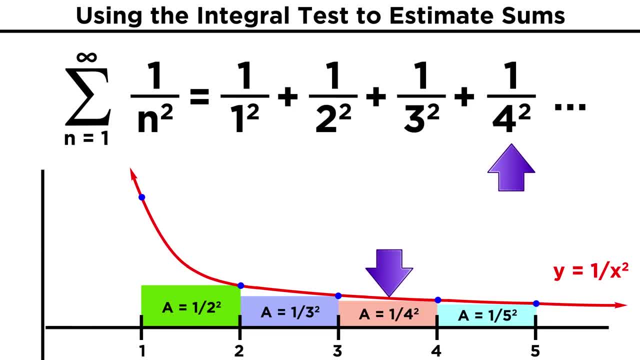 is one over three squared. So every rectangle, all the way to infinity, has a corresponding term in the series, and we are leaving out only the first term, one. The sum of the areas of these rectangles is pretty close to being area under the curve, which we know is just the integral of the function. 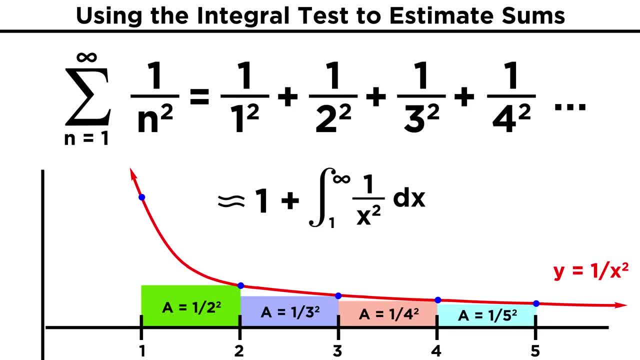 So the sum of the series will be approximately equal to one, to account for the first term in the series that has no corresponding rectangle, plus this improper integral, which approximates the sum of all the rectangle areas and therefore accounts for the rest of the terms in the 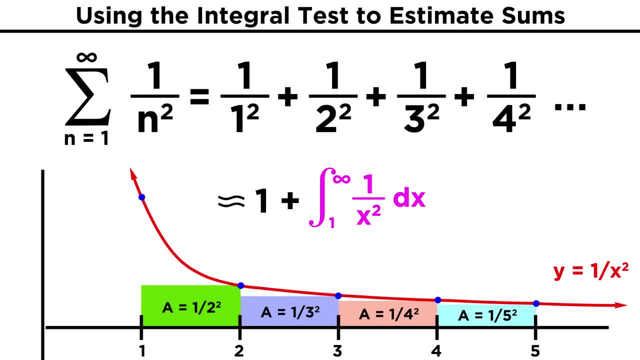 series. We know how to evaluate the integral. we just find the antiderivative, which is negative, one over X, And we evaluate at infinity and then at one which gives us zero minus negative one or positive one. The one from before plus the one from the integral equals two. so that's our estimate. 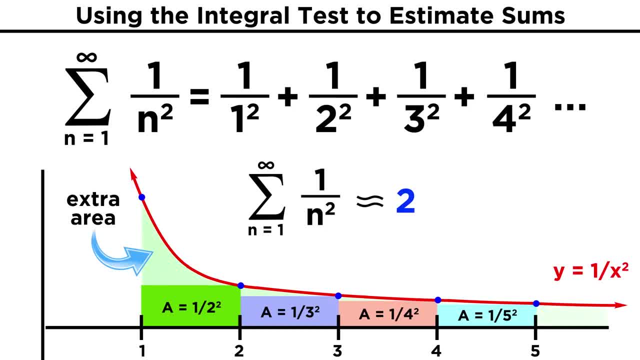 for this sum. Now we know that the rectangles don't quite match. They don't quite fill up the total area as there are some empty spaces. so the integral is bigger than what we really wanted and therefore the actual value for the sum of 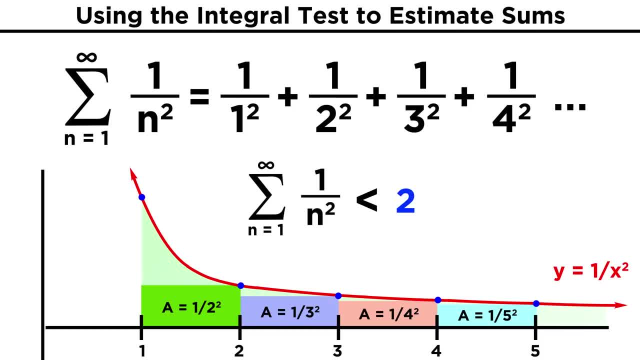 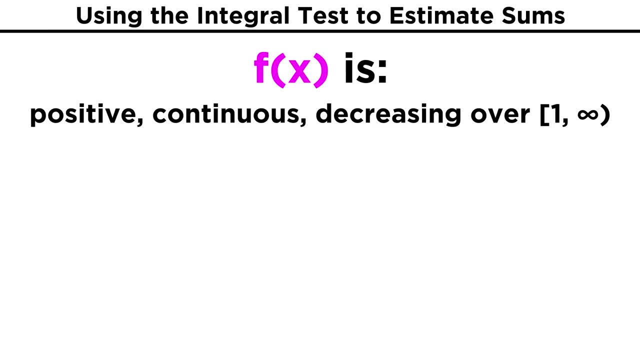 the series must be a little less than two, But we've still done a pretty good job at getting some information about the series. How can we summarize this technique? in a general way, We can say that if we have some function, F that is positive can be multiplied by. 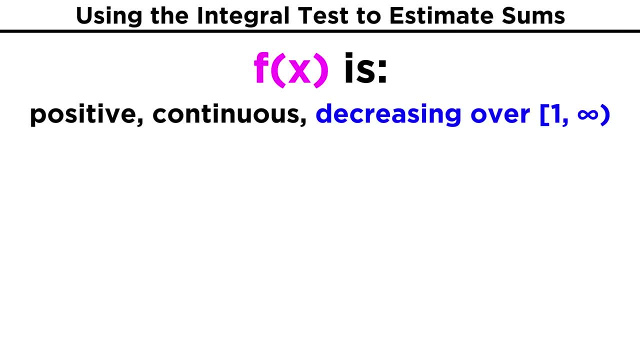 infinity, continuous and decreasing from one to infinity, and we also have a sequence that is derived from this function, in other words, A sub n equals F of n. then the series that can be formed from this sequence, from one to infinity, will be convergent only if 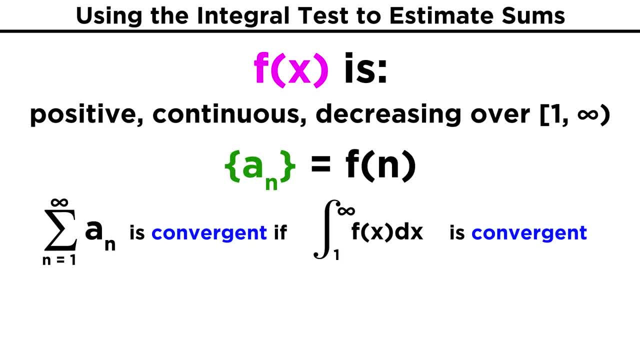 the corresponding improper integral is convergent. If the integral is divergent, the series will be divergent. If the series is indeed convergent, then we can also estimate its sum by calculating the improper integral in some way that is similar to the example we just performed. 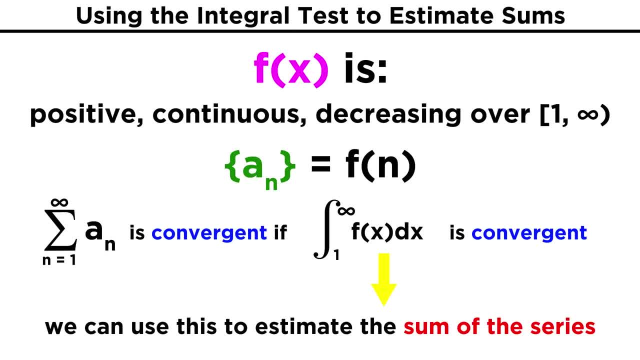 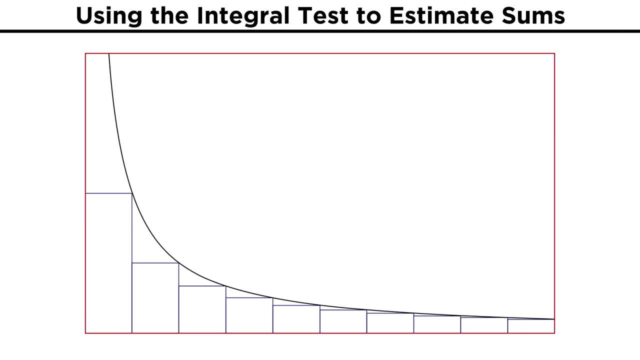 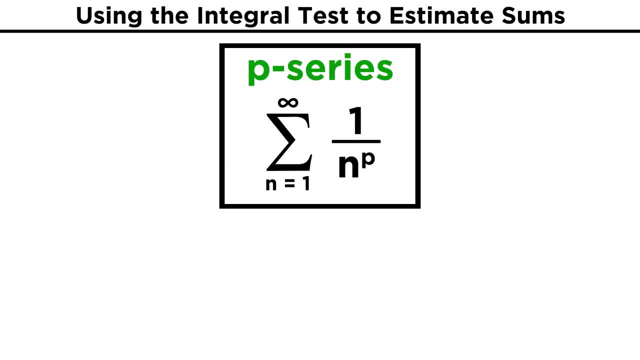 And that is the essence of the integral test. Let's just mention a few important truths that can be found by applying the integral test. Any series in the form of one over n raised to six To some exponent is called a p series. This includes our first example: one over n- squared. 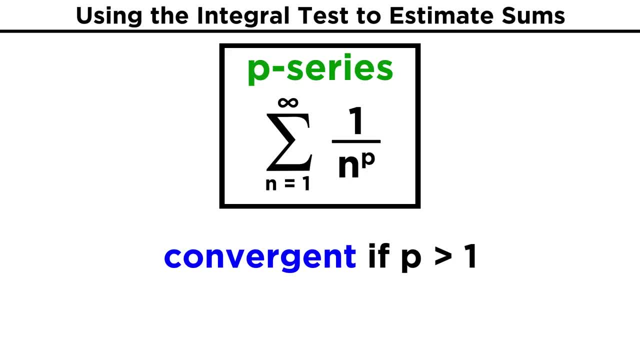 As it happens, any p series will be convergent if p is greater than one and it will be divergent if p is less than or equal to one. So if we have one over n cubed, it will converge. If we have one over the cube root of n or one over n to the one third. 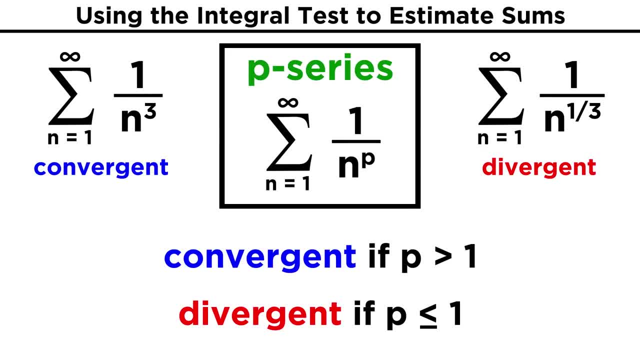 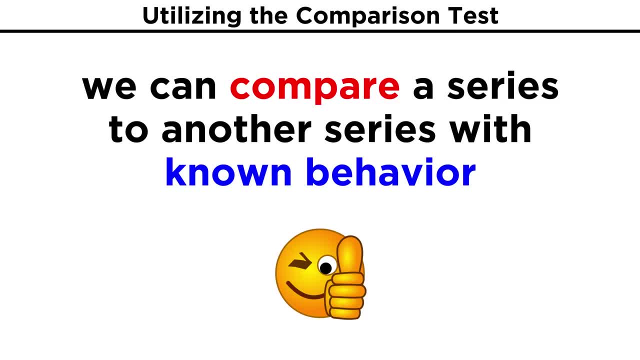 It will diverge. There is one more test we can learn. that will be an important technique and it is called the comparison test. With this technique, we will take some series and compare it with a similar series that we know to be convergent or divergent. 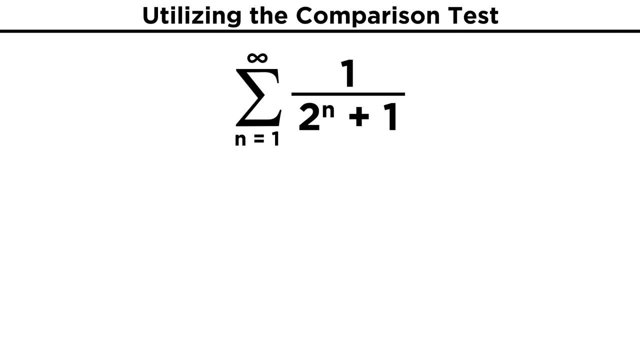 For example, say we are looking at the series one over the quantity, two to the n, plus one from one to infinity. This looks like it could be tricky to assess, but what if we compare it to a simpler series one over two to the n? 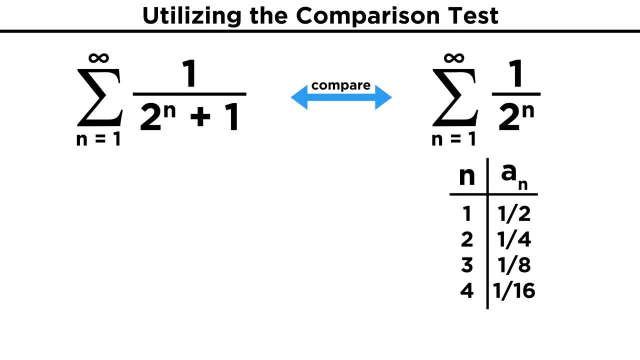 This is a simple geometric series and, as we have already seen, the fraction gets smaller and smaller as the exponent gets larger and larger, so the sequence converges to zero and, as we saw in the previous tutorial, this is indeed a convergent series with a sum that 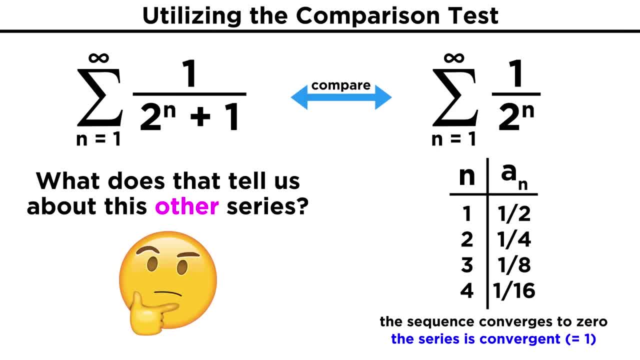 is equal to one. If we know that this series converges, what can we say about the original one? Well, this plus one term in the denominator means that each term in this series must be smaller than each corresponding term in the other series. and if every term is smaller, 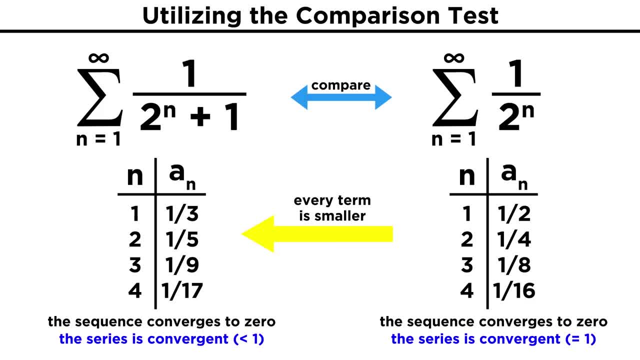 then this series must also converge and the sum of this series must also be less than one. So we aren't calculating the percentage of the sum. That's it, Thank you. precise sum with the comparison test, but it is a useful tool for determining whether. 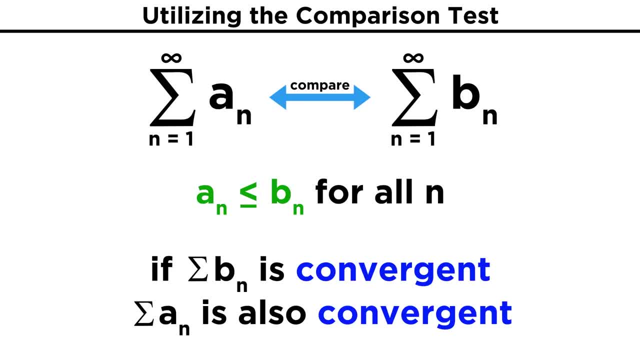 a series is convergent or divergent. If every term in a series is smaller than each corresponding term in another series- that is known to be convergent- then it too must be convergent, as we just saw. On the other hand, if every term in a series is larger than each corresponding term in 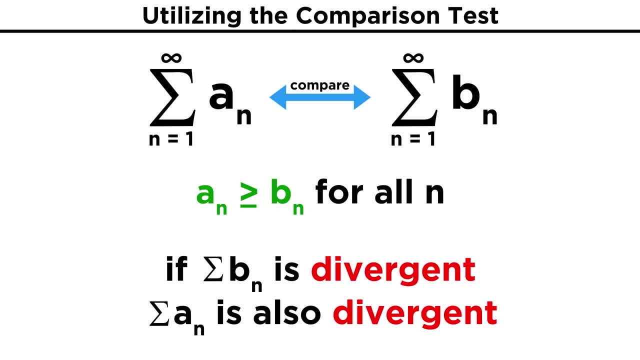 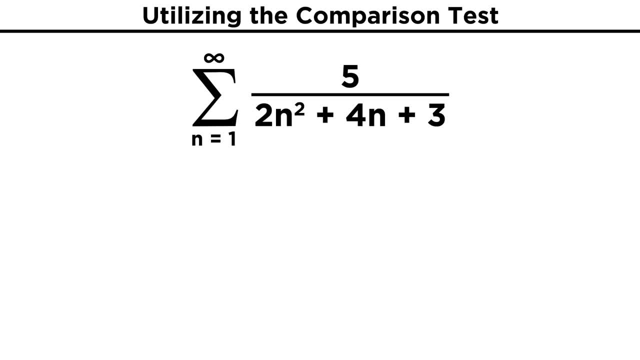 another series that is known to be divergent, then it too must be divergent. Let's just do one example to make sure we can apply this. Take the series five over the quantity two n squared plus four n plus three. We can simplify this to: five over two n squared. 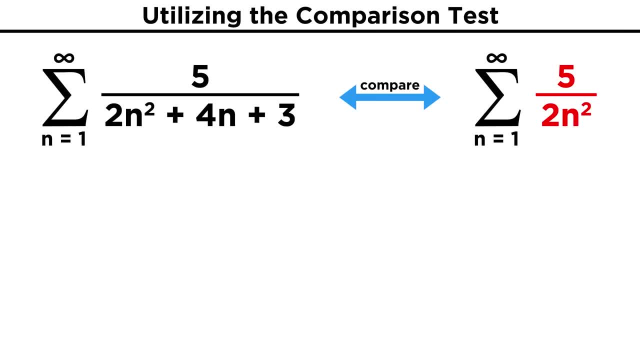 What do we know about this simpler series? Well, we can manipulate series just like we do integrals, and five halves is a constant that can be pulled outside of the sum, as doing this is essentially like factoring five halves out of all the infinite terms in the series. 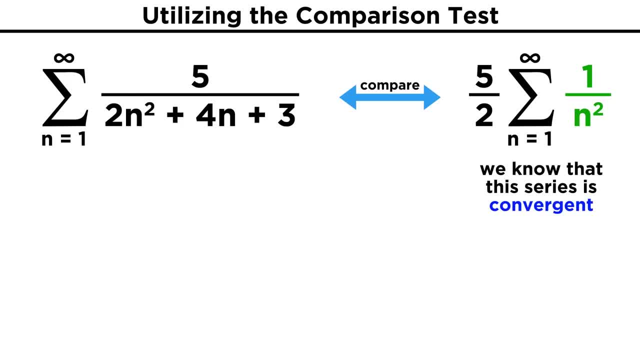 Then we are left with something very familiar and we know that this series is convergent. Our original series has terms that must be smaller than the terms in this series, because there is more in the denominator and n is always positive, so the fraction is always. 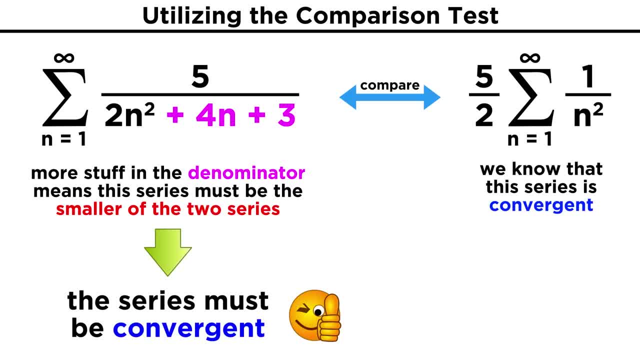 smaller than if those terms weren't there. Therefore, this series is also convergent, and its sum must be less than that of the one we are comparing it to, Now that we have the basics down for assessing whether a series is convergent or divergent. 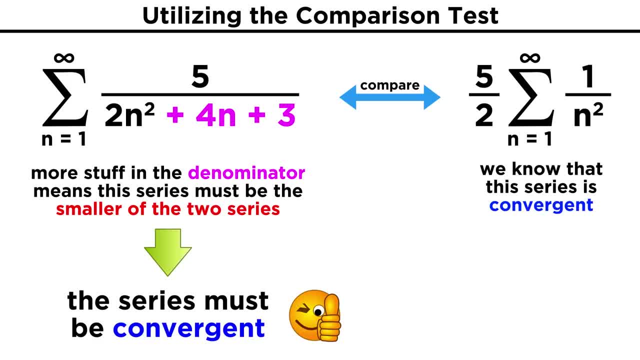 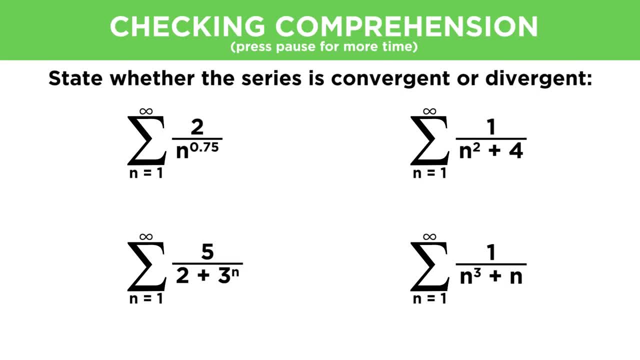 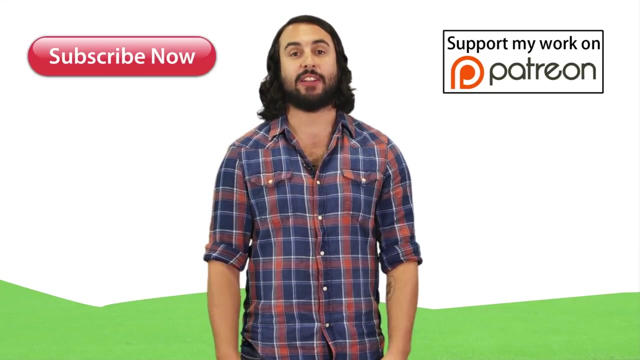 let's go back to our original series. Let's check comprehension. Let's check comprehension. Thanks for watching, guys. Subscribe to my channel for more tutorials, support me on patreon so I can keep making content and, as always, feel free to email me professordaveexplains at gmail dot com. 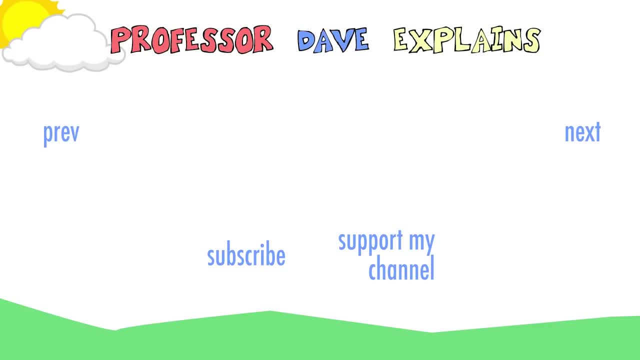 I'll see you in the next one. Bye.